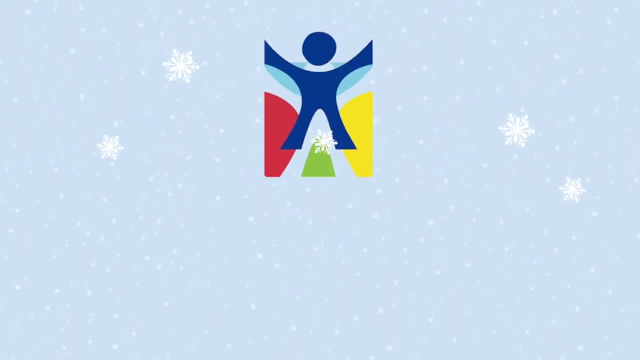 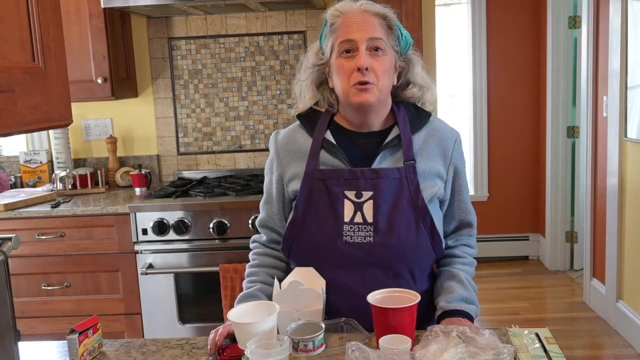 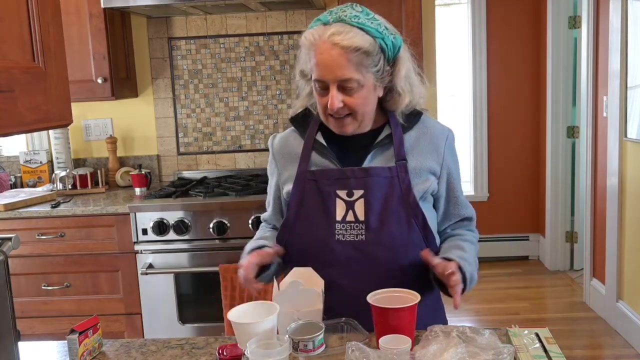 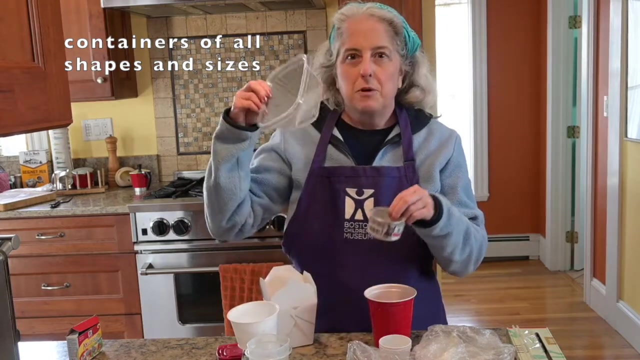 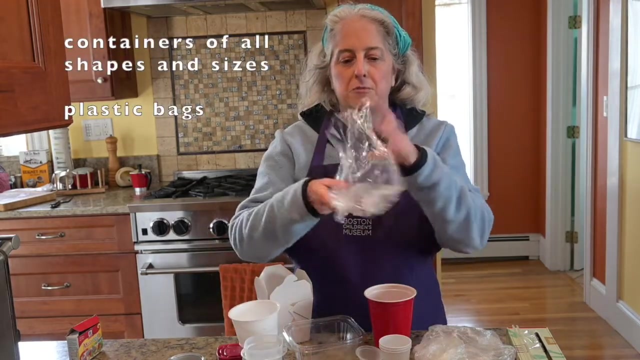 This is a great activity because you can go as crazy with it as you want. Here's what you'll need: Containers. Containers of all different sizes and shapes, and from your recycle box or maybe some storage containers that you have, You can use plastic bags, anything that will hold water. 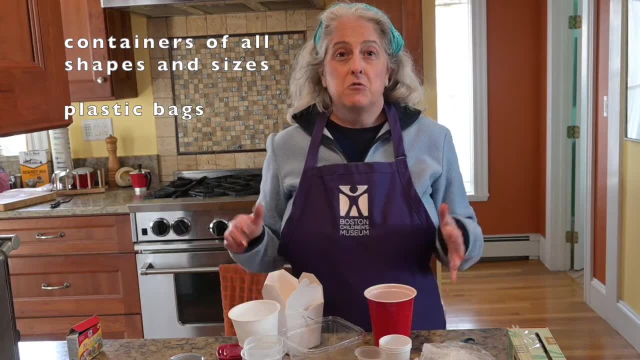 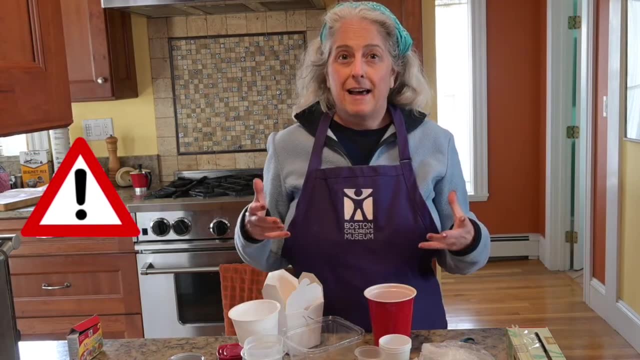 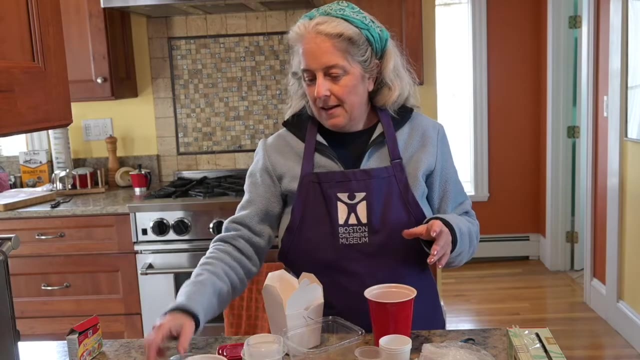 Now, one thing to keep in mind is you don't want to use anything. that's really important, because sometimes the ice can crack a container. So definitely don't use glass and definitely don't use your, your favorite little plastic bin If your containers have lids. 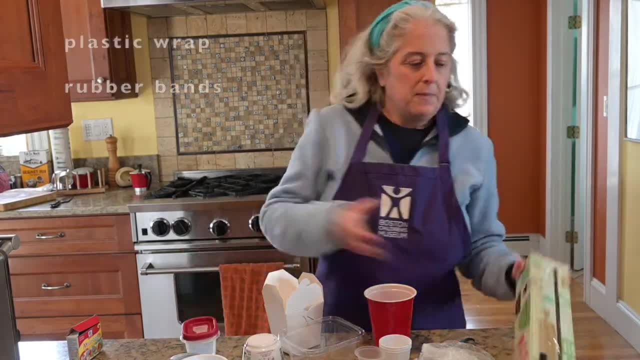 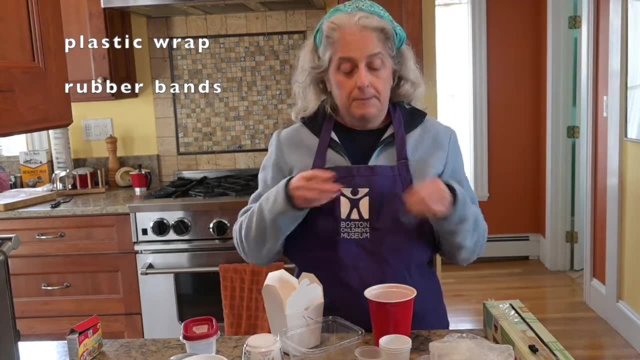 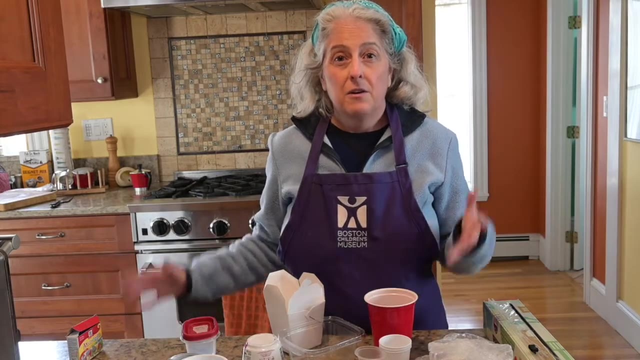 you can use them. These are in a great condition. but if they don't, you'll just want to cover it up with some plastic wrap and then hold that on tight with a rubber band. You can fill your containers with just water and put them in the freezer and leave it at that. 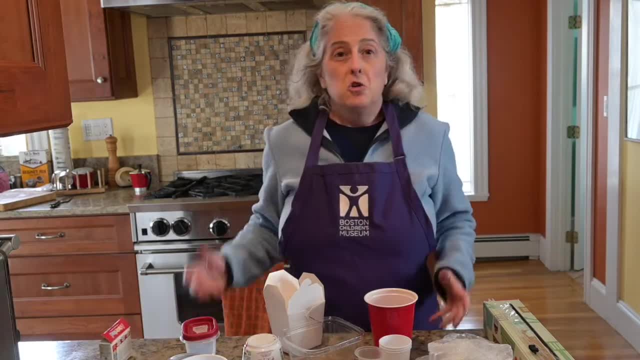 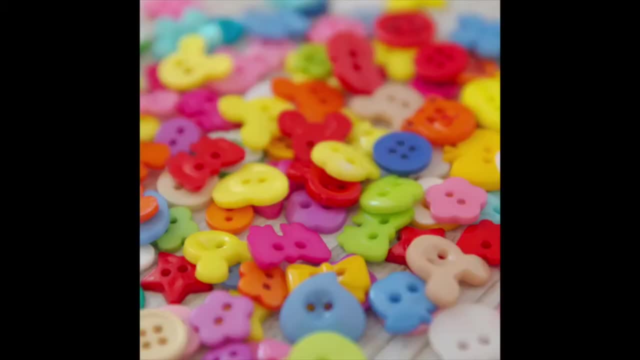 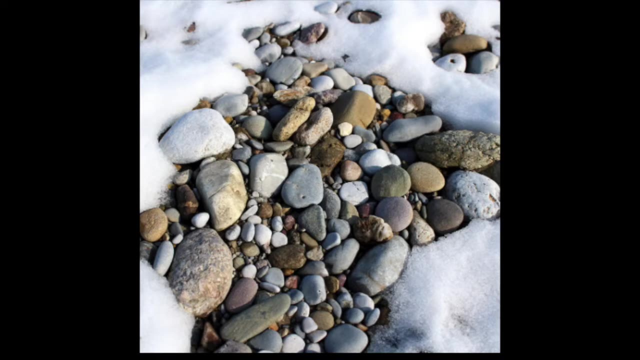 Or you can try putting some food coloring in there. You might also want to try putting some or other small objects inside your containers, or go outside and collect some interesting-looking leaves or other things from nature. Whatever you can think of, you can put it in your containers. 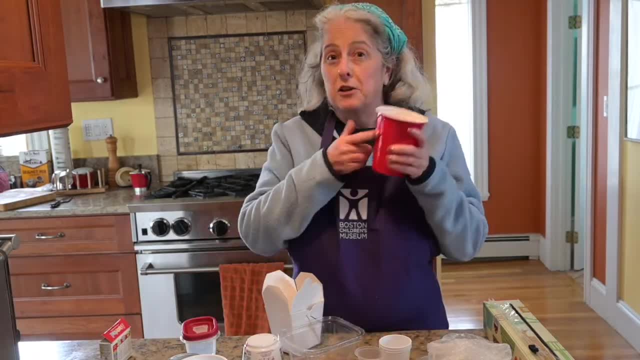 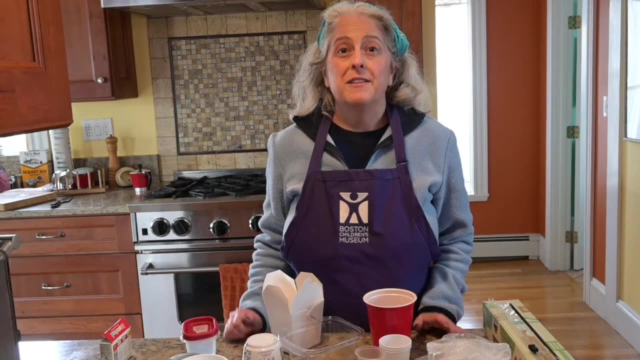 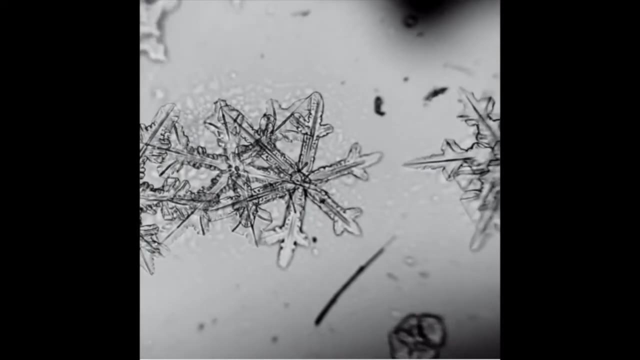 Fill them up with water as much as you like. You don't have to fill it all the way to the top if you don't want to, And then put them in the freezer for a few hours or even overnight, Well, my ice blocks are frozen. 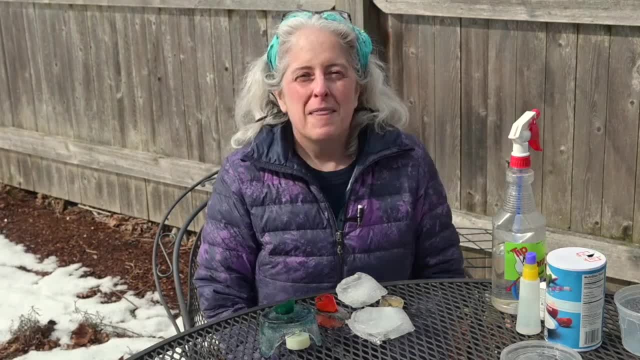 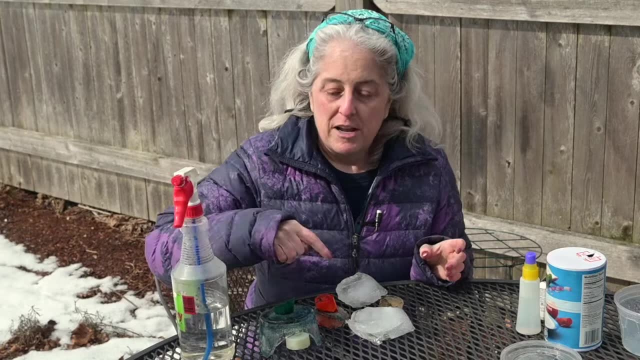 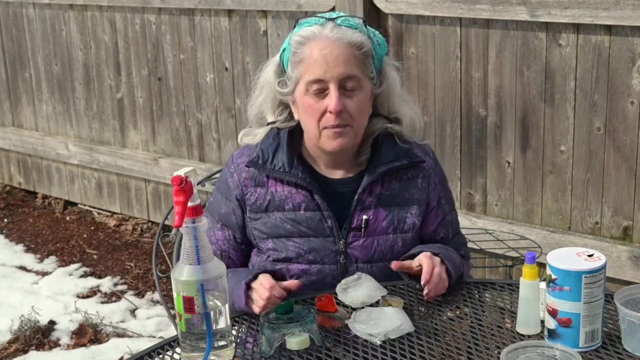 and I got them out of the containers that I froze them in. That was a little challenging. I tried taking a spray bottle of warm water and spraying it around the outside of the containers to loosen up the ice. Then I whacked it on the ground a couple times and the ice came out. 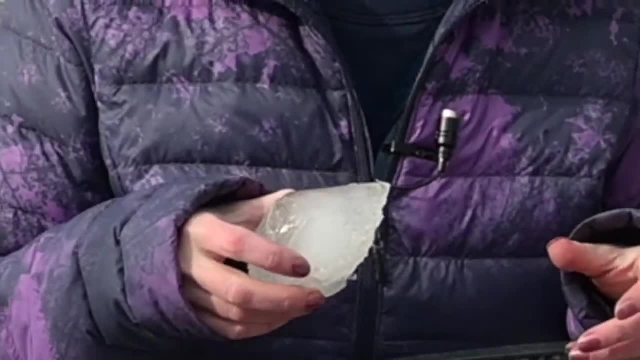 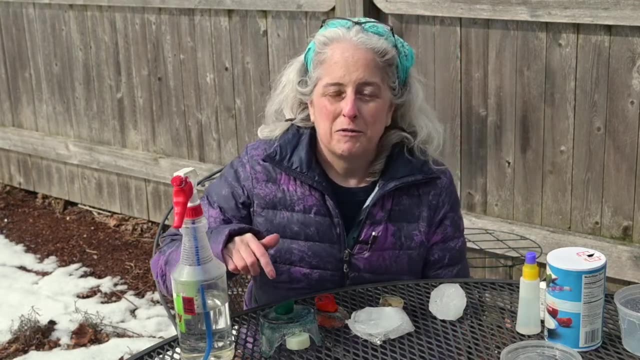 For the ones that were in the plastic bags. I just peeled the plastic bags away and now I have these rotting, really weird shapes On this one. I don't know if you can really see it, but the ice broke as it was coming loose from the container.